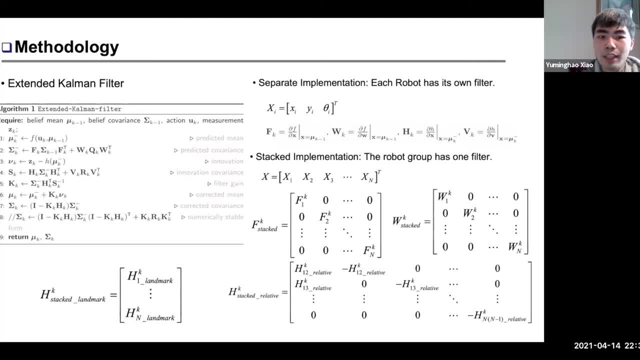 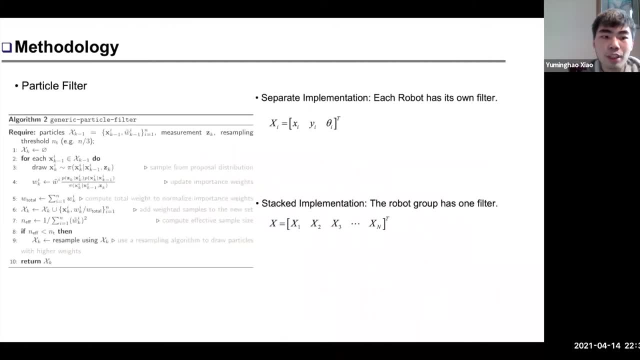 are calculated individually. Another way is to stack all states in a robot group into one matrix, and the equations for stacking the Jacobians are also listed here. in the second block For particle filters it also has two implementations: separate and stacked version For implementation. 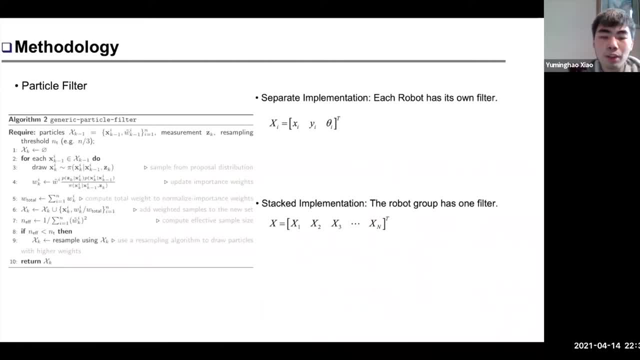 from implementation point of view they are pretty similar, but in terms of computational cost there are some obvious distinctions between the two. For example, for a particle filter, a particle filter is the same as a particle filter. For a particle filter: 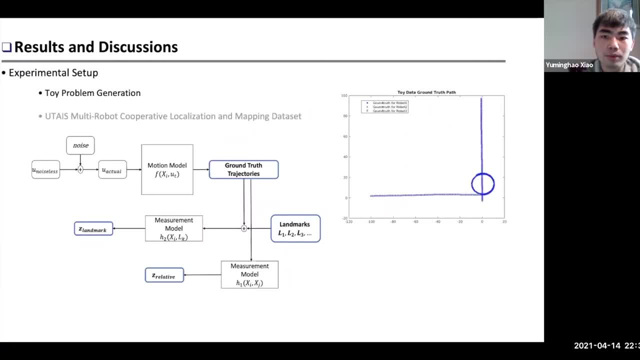 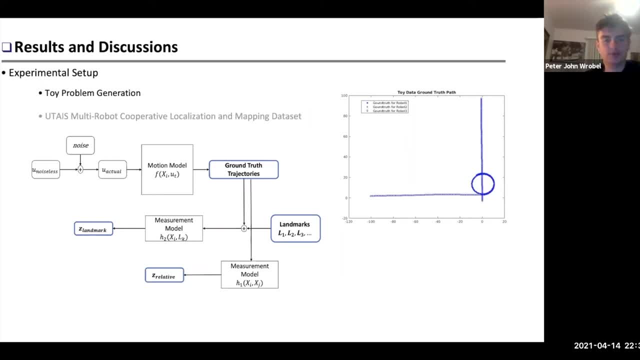 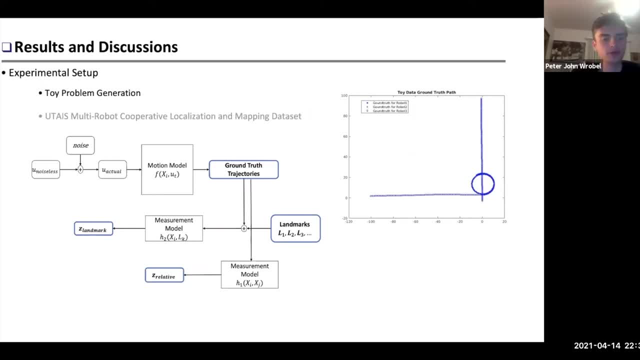 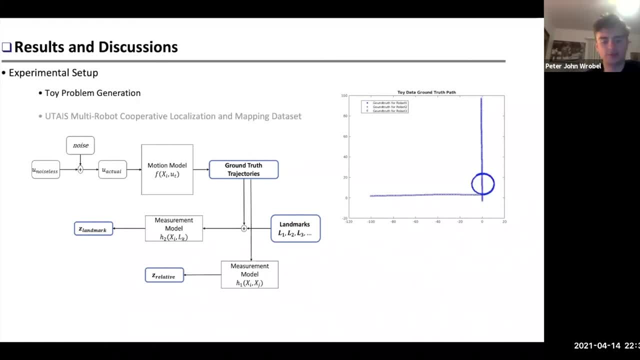 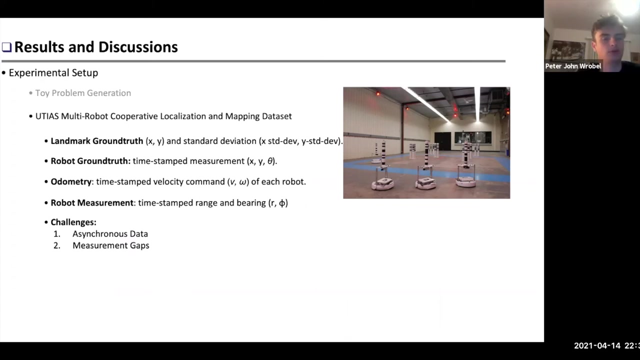 For a particle filter. a particle filter is the same as a particle filter. Before we get to outを and when I 天 th t e t using the UTS multi-robot cooperative localization and mapping data set. The data set provides IMU measures for the odometry and then also provides measurement values by having robots look for. 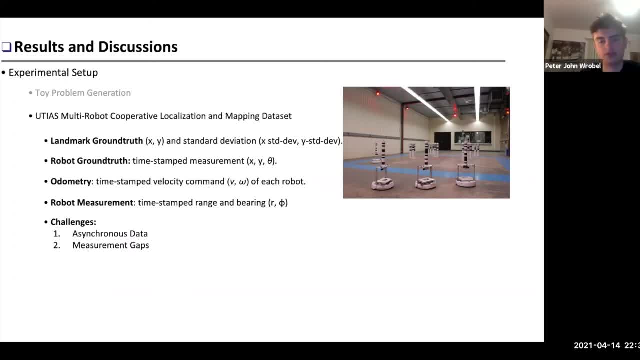 barcodes while they're traveling, and they can pick up barcodes off of landmarks and also off of each other. Hence we get both landmark measurements and relative measurements. The challenge provided by this data set is that the data is not synced with respect to time, So we had to make sure that. 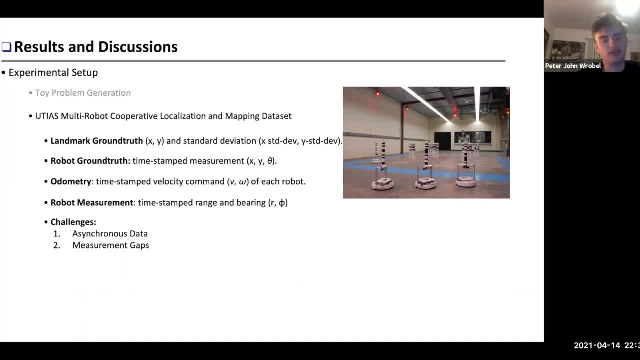 the odometry and the measurements were synced in time. And then also there are measurement gaps. For example, if a robot's facing a wall, it's not picking up any barcodes, So there's intervals of time when we don't get any measurements, basically making batch updates impossible. 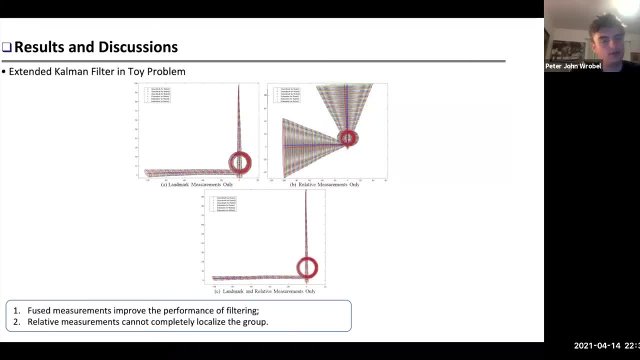 Looking at our results, we see that the EKF performs well for the toy problem. just using landmark measurements, And then using only relative measurements, we get a good body frame estimation or good orientation. However, it's not accurate in a world frame, as we don't have a world. 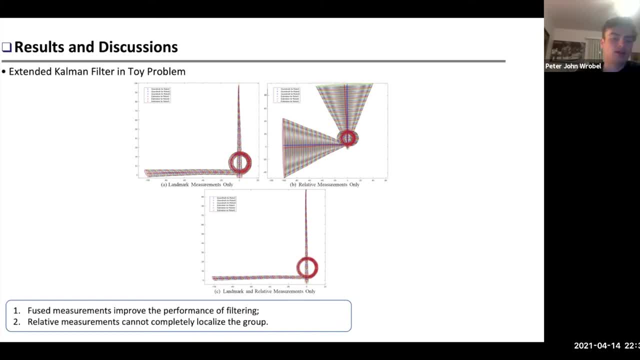 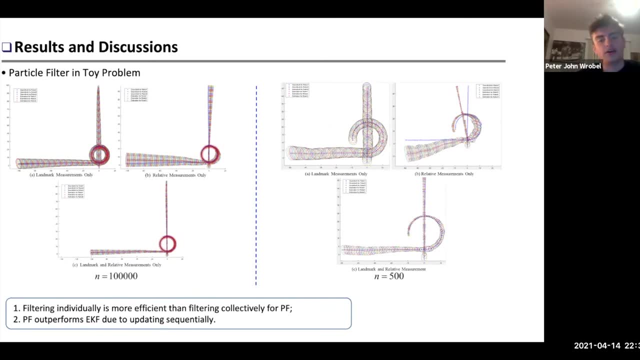 frame reference. However, combining the two measurements, we see we get not only good estimation but a lower variance. This holds also for a particle filter, as seen here And on your left you've got the stacked particle filter and then you've got the individual particle filter With the stacked. 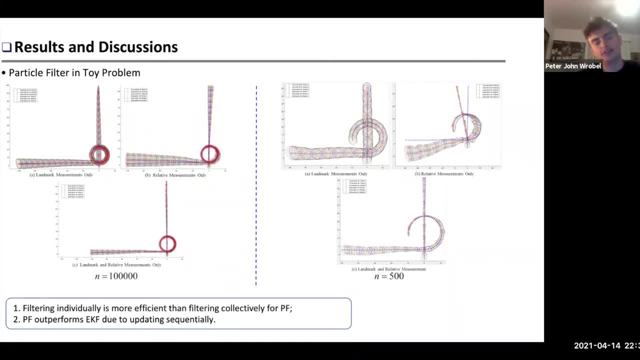 particle filter and the individual particle filter, we get very similar performance, where the combined measurements outperforms the landmark measurements. However, with respect to computation time, the individual one runs significantly quicker. In this image, we're only using 500 particles per filter instead of the 100,000 total for a stacked one. 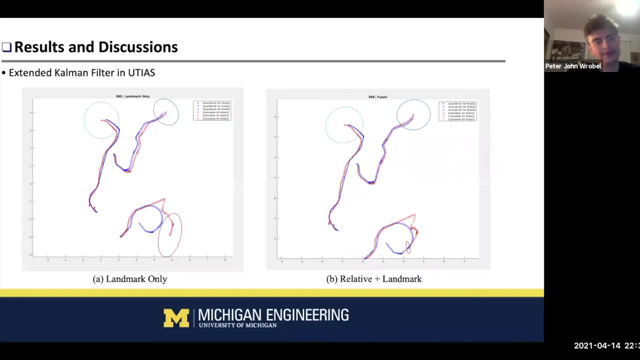 In this image we're only using 500 particles per filter instead of the 100,000 total for a stacked one. Now, applying these filters to the real data set, we see a very similar performance. For example, here we apply the EKF on one of the data sets provided by UTS and we see that with landmark only we 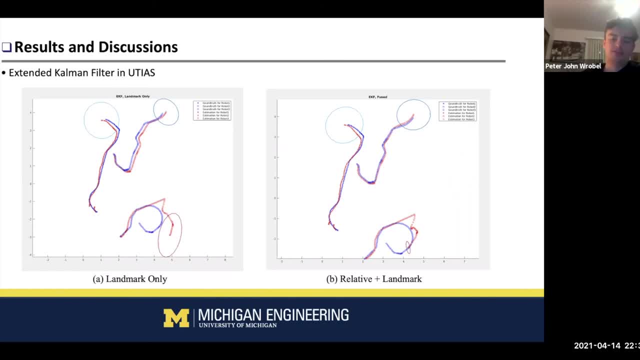 get pretty good results, but adding on top the relative measurements, we get an even better result, especially for the robot right on the bottom there. Yeah, so that holds for both EKF and particle filter. The paths are very similar. They're not the same. 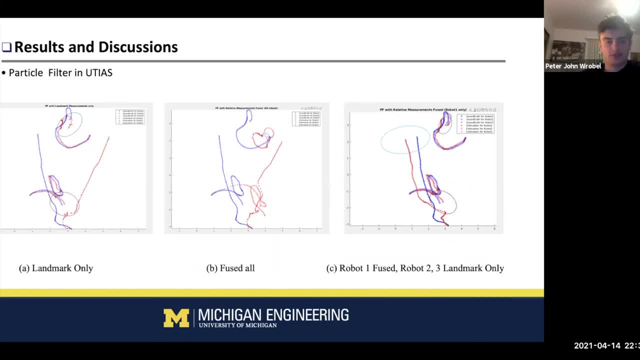 They're the exact same. So, for example, if you have to generate a new filter, for instance, we have a filter with the same activities- particle filter- and the paths are virtually indistinguishable. However, there is a data set that has an outlier- this one right here. As we can see in figure A, two robots are well estimated. 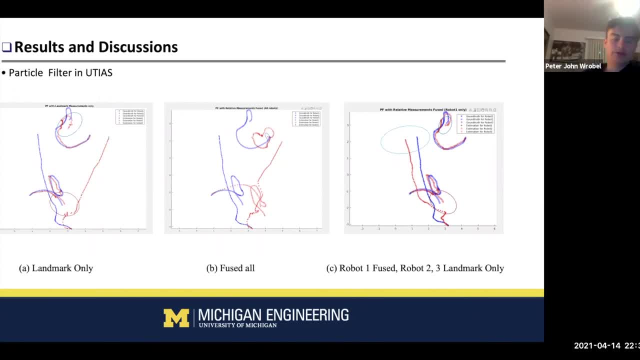 by landmark-only adjustment, while one- the straight line- we'll call robot one- veers off significantly. If we blindly apply relative measurements to all three robots, that error is propagated to both of them and then causes all three robots to have a poor estimation. 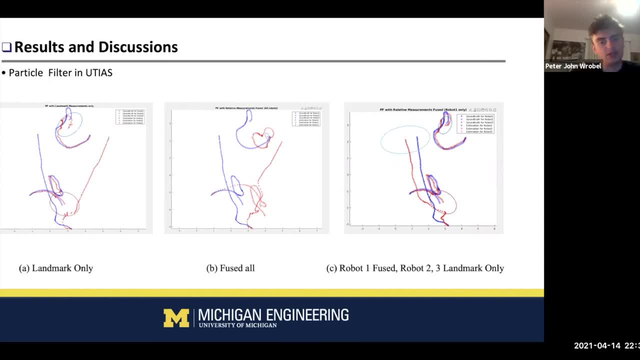 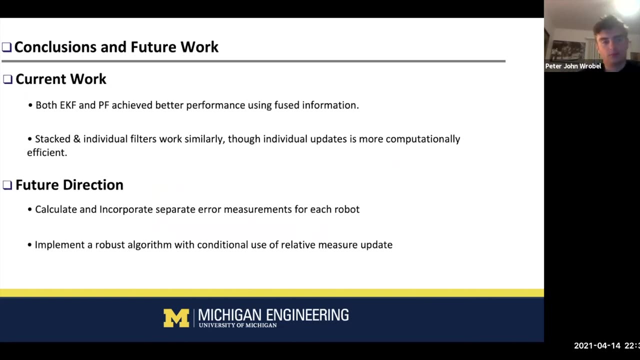 However, if we smartly apply only relative measurement adjustment to the straight line robot one, we see that the other two robots keep a good shape and robot one gets better adjusted. So from our current work we saw that both EKF and PF achieve performance In most cases. 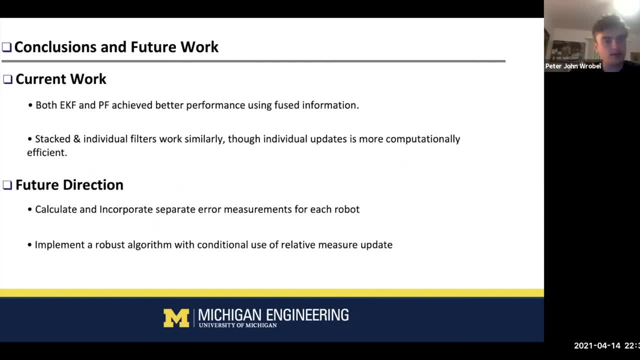 that's better when we fuse the information And they both perform similarly very well. And in case of the stacked and individual filters, they also work almost the same. However, in the case of PF, an individual update runs significantly quicker. Looking onto the future, we have a lot of information about the future of the robot. 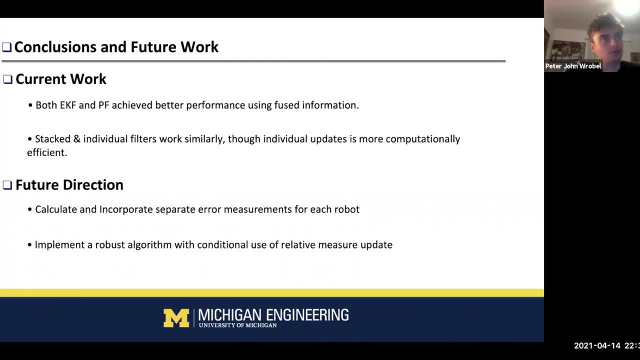 We'll want to make sure we find the right noise for each robot, because right now we're assuming each robot has the same noise And we want to figure out a smart way to figure out when to apply the relative measurement update, because we saw in that one case it could mess everything up. Thank you.